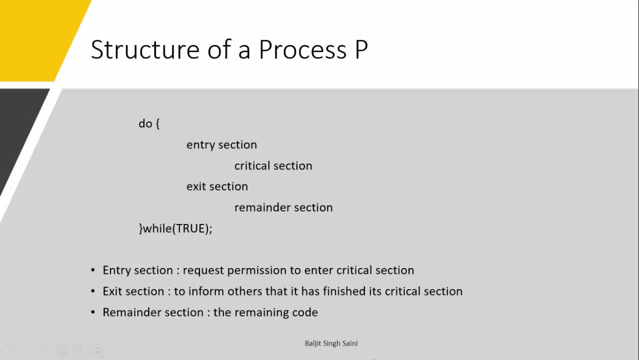 it should satisfy this overall structure of a process. so our code we will introduce a entry section. entry section is that portion of the code in which the process will request to enter the critical section, entry section, portion over critical section, if the request is granted or if it is able to. 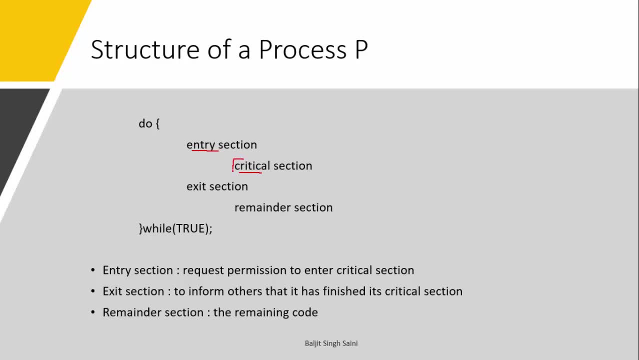 enter the critical section. so whatever lines are in the critical section will be executed. once the critical section is executed, critical section polar portion would execute over here. then there will be a exit section. what will be there in the exit section? the exit section will contain some lines of code which will inform others that the process is out of the critical. 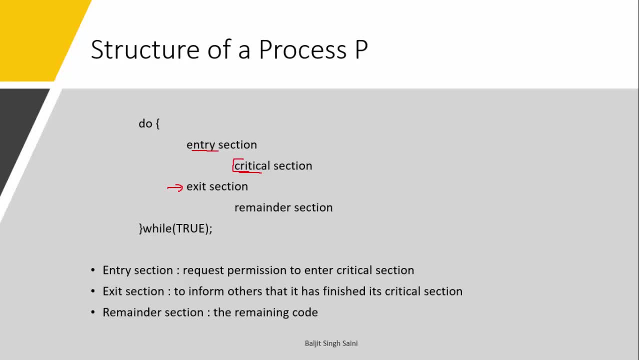 section, and if any other process wants to enter the critical section, than it can do so. so what you have to do in the exit section is to the other process. the signal has to be garden process and the current process is out of the critical section. and if any other, 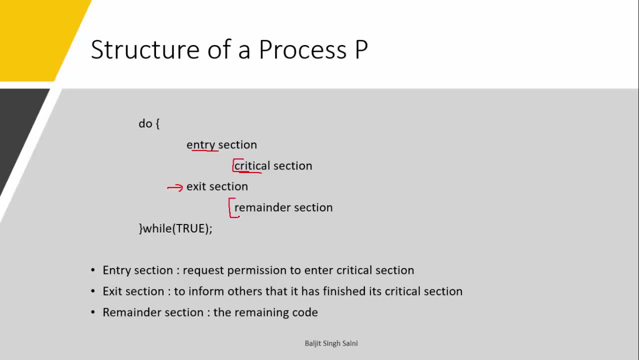 critical, there is free to do so. that's what we call the rest code, remainder section. so you have to take care that what you provide, the solution, is before critical section. you should also авit unit neutrality should not be that such that first time you have to do critical section then it is free to dude series. the rest of the code is it a paper to asaliind connecting the semesters? that the main intersection time, the rest of the code is what is known as remainder section. team the code is calledбы mandatory section. then you have to keep an eye on this. so if you keep a solution by now, then one of these solutions should not bealle likely to have a solution after that. then you will get in place critical section. then it this is pursuing security system. first you will require that part of the section. 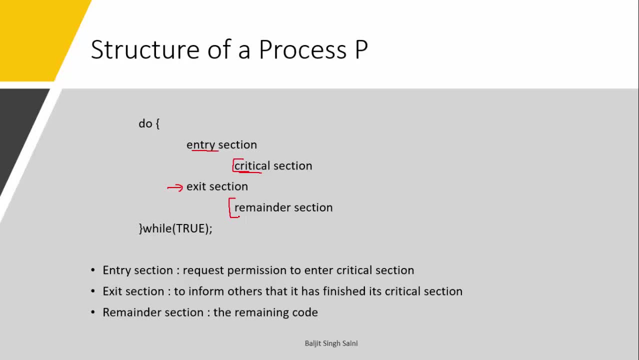 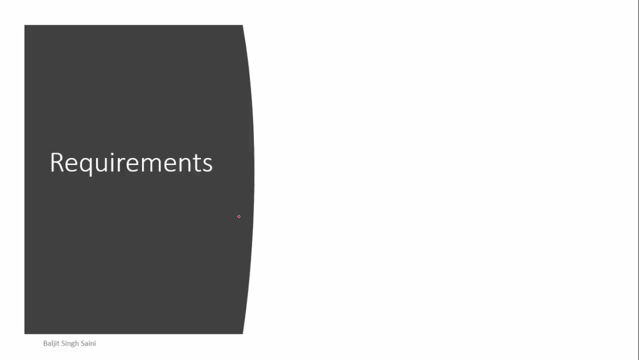 Whatever solution you provide, you have to introduce a section before the critical section, which we will call entry section, and exit section after the critical section. Now, whatever is the solution proposed, it should satisfy three things. It is compulsory to satisfy three requirements for each solution. 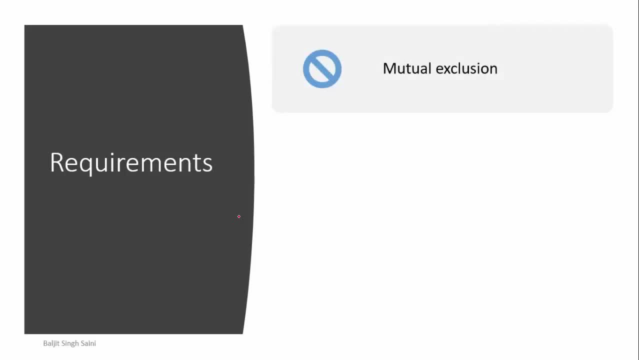 The first requirement is mutual exclusion. Mutual exclusion means that only one process can be in the critical section at any given time. What is mutual exclusion? Mutual exclusion means that at a time, only one process can run in the critical section. Second is progress. 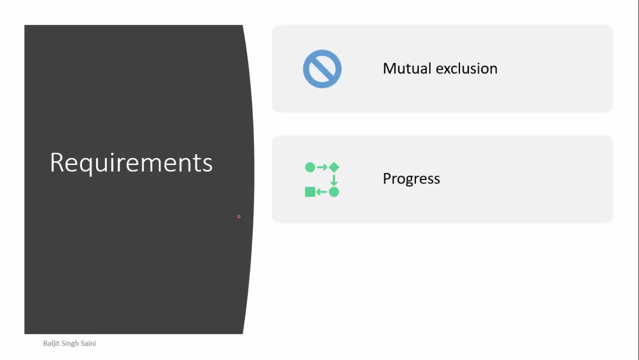 Progress means that system should not halt. Let us suppose that more than one process are entrusted to enter the critical section- Exit section, Then at least one of them should be able to do so. Progress means that one of them should enter the critical section. 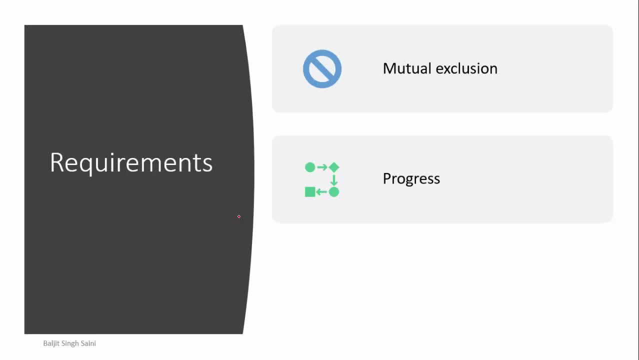 It should not happen that all are waiting for others to do so. One process is waiting for the other, the other is waiting for the third, the third is waiting for the first and no one enters the critical section And all three are stuck. 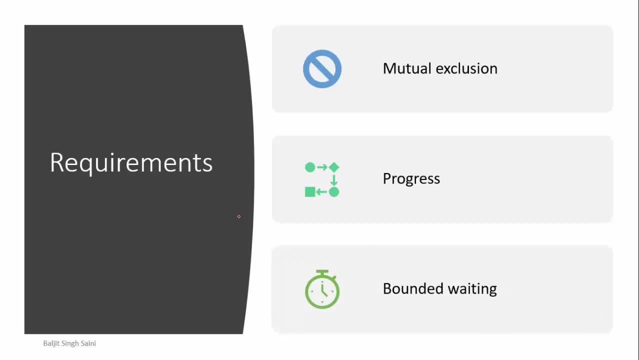 It should not happen. Last is the process. Next is bounded wait. Bounded wait means that if a process has requested to enter the critical section, after that request there should be a time bound. After that its return is compulsory. Let us suppose that there are three processes: P1, P2 and P3.. 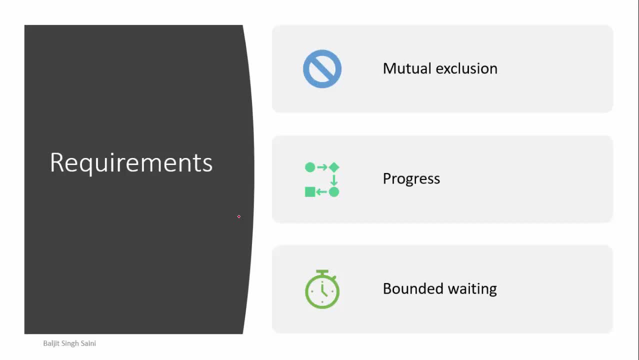 All want to enter the critical section. P1 made a request at time. t is equal to zero, But the request is granted for P2.. P2 is allowed here, Then we allow P3. But P1 is still waiting. So before P1 gets its turn, P4, P5 process has come. And they also want to enter the critical section And rather than giving turn to P1, we allow P4 and then P5. And P1 is waiting again. So this should not happen. There should be an upper bound: After how much time or after how much process the turn of P1 has to come to enter the critical section. 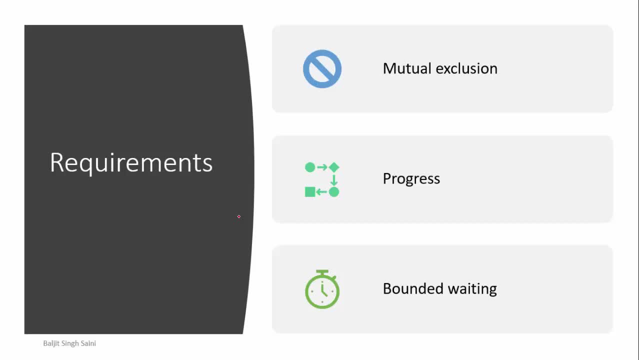 It should not starve. So these are the three requirements. They should be met by any solution to the critical section problem. Now what generally happens is in your exams or in the exams like GATE or UGC NET. They give you a solution and ask which of the requirements is not satisfied. 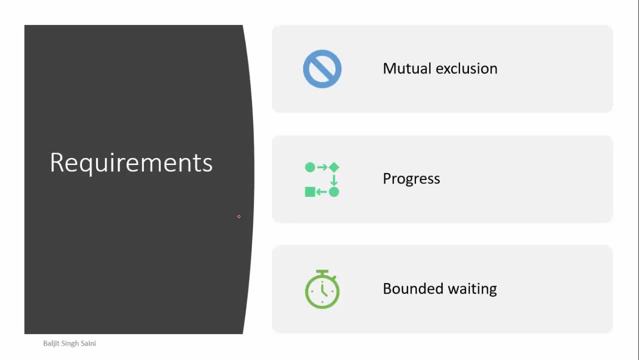 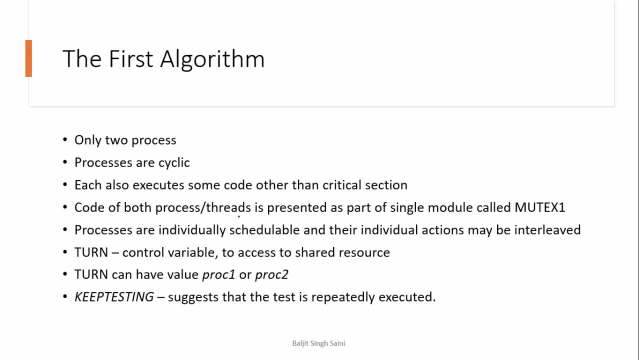 So they will give you a question and will ask you which requirement is not satisfied. So we are going to discuss two such solutions. This is how the question comes in the exam. So let us suppose that there is a solution. This is the solution. 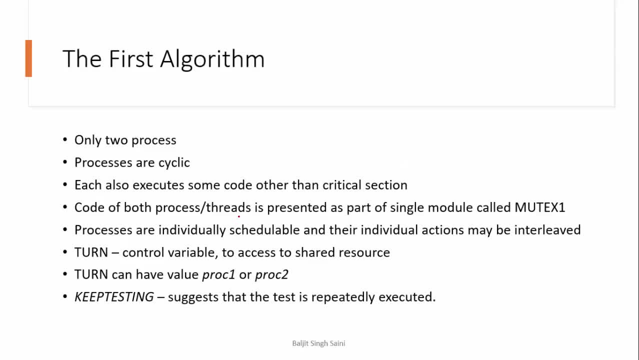 So I will just explain how it works. Now. the solution is for two process only, And we assume that the process are cyclic: First P1 goes, then P2,, then P1,, then P2, and so on. Both the processes execute some code other than the critical section also. 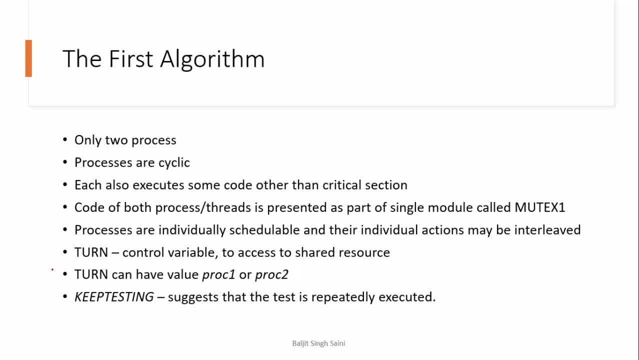 Now there is a variable turn which controls whose turn it is to execute into the critical section. So the turn variable can have two values: Process 1 and process 2.. There will be a term keep testing, which means that the condition should be tested again. 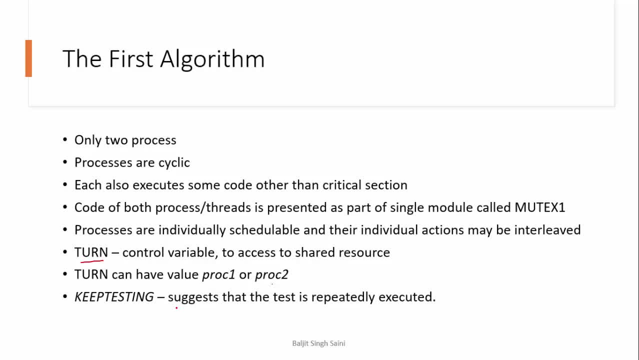 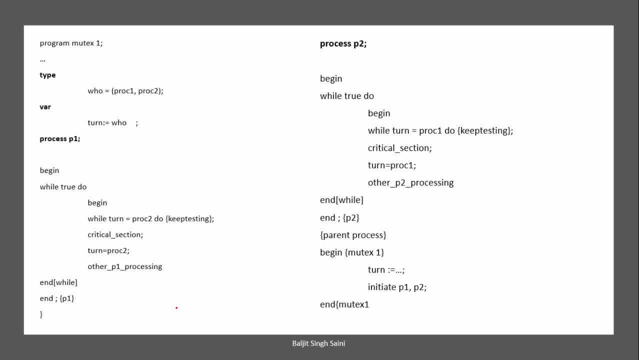 by the process. So we will just look into the code and all this will make sense. The code of the process is same. The code which is in P1 is in process P2.. Just the variable: where process 1 is there, process 2 will happen. 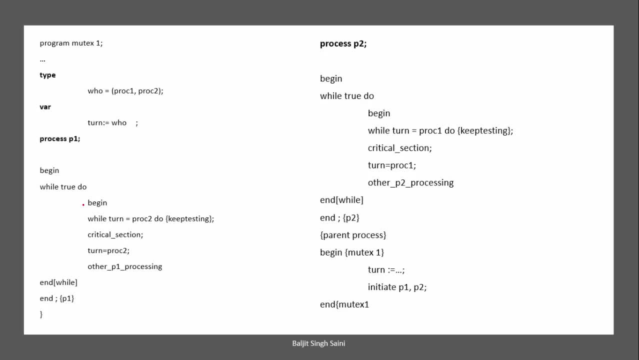 Where process 2 is there, process 1 will happen. This is where you need to work. This is the main part. Now, this is the entry part. At entry part. what is the entry section Before the critical section? It will check. 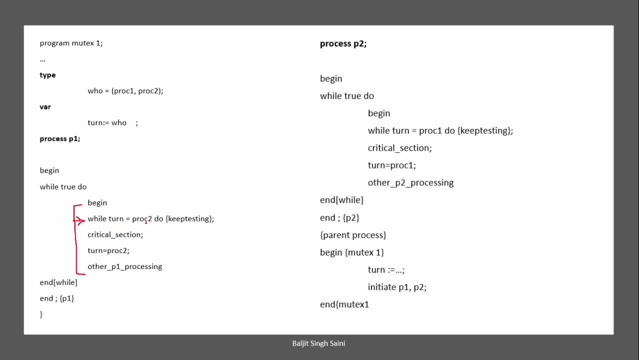 This is process 1.. So it checks, while turn is equal to process 2.. Turn is a variable. What can happen here? Either process 1 or process 2.. So what did process 1 check? Is the turn of process 2?? 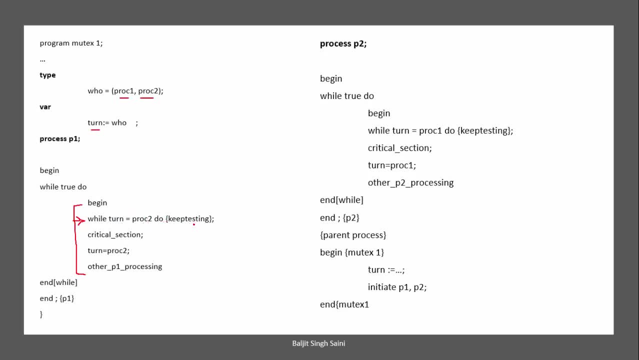 If yes, then do what? Keep testing. Keep testing means you keep checking What is the turn of the process And if the turn is not, of process 2. This condition is false. What will happen? It will come out of the while loop. 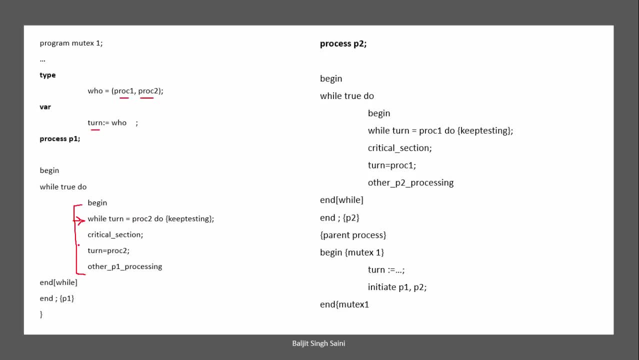 And then it will enter the critical section. After the critical section there is exit section. What to do in the exit section? What did it give the turn To process 2.. So P1 itself will give the turn to process 2.. 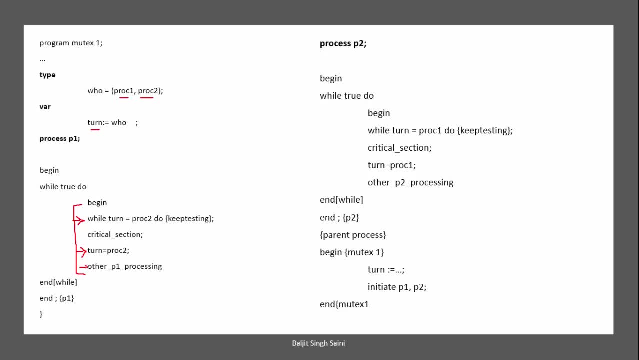 Okay, And this is the remainder section, That other P1 processing, Other P1 processing means the rest of the code. Okay, So what will process? do It will check first. Is the turn of the second process? If yes, then keep testing. 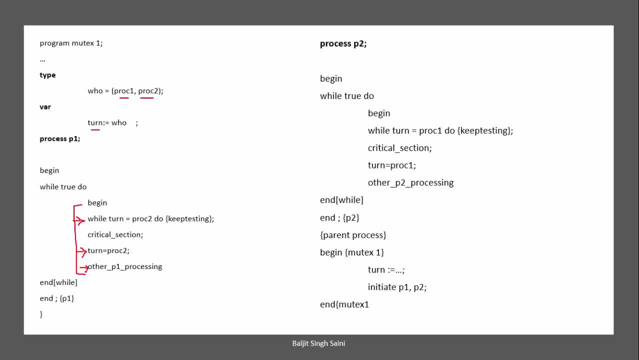 Otherwise, enter the critical section. After coming out of the critical section, it is going to give the turn to another process. If you see the code of the second process, it is the same, Just the change of variables. Now, initial value of turn: you need to set it. 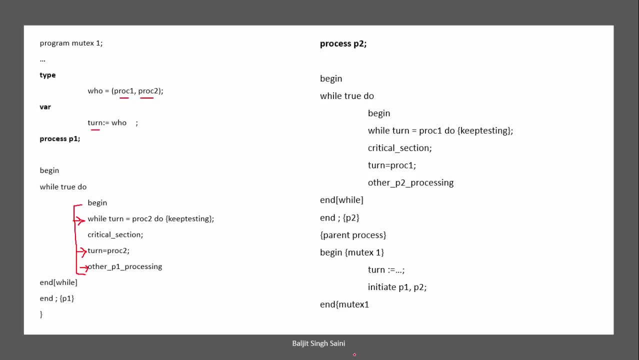 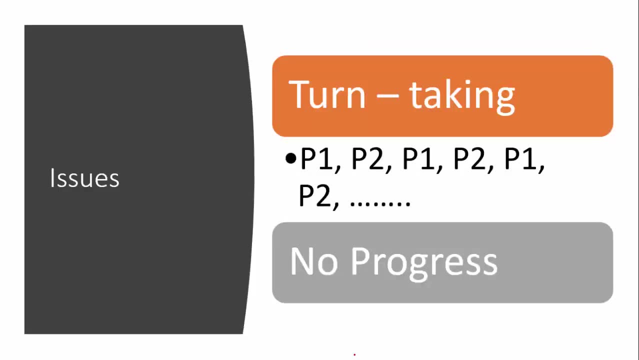 Either we have to give it to process 1 or to process 2.. Okay, Now what will be the issues with this? You need to tell now. The first issue is that it is a turn taking kind of an algorithm. First, let us suppose if the turn of P1 was before. 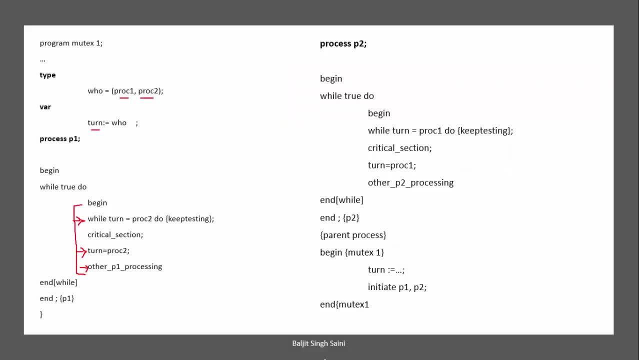 So P1 will assign this turn to process 2.. So the second turn will come to process 2.. Process 2 will assign this turn to process 2.. Okay, P1 will assign this turn to process 1, and so on. 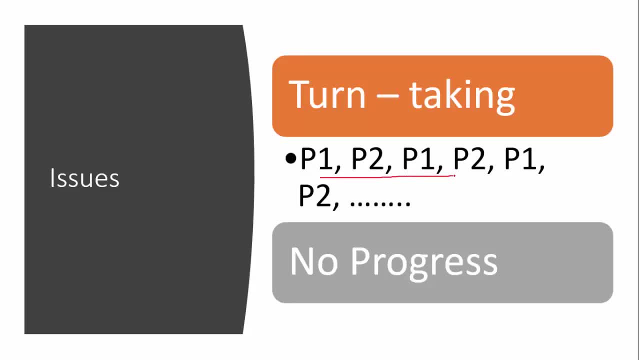 So they will be taking turns P1, P2, P1, P2.. P1 will not be able to run twice because the moment it comes out of the critical section it gives the turn to process 2.. What will be its condition? 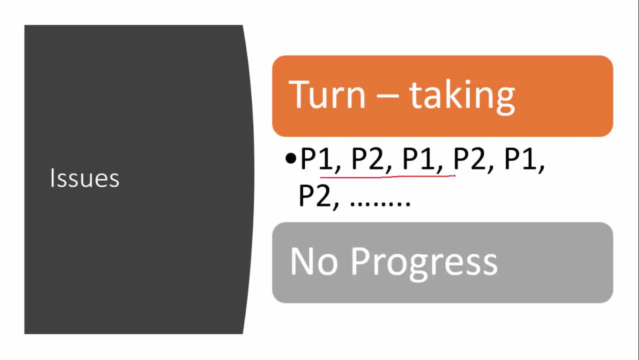 It will be true, It will not be able to enter itself. Second, it does not ensure progress. This is the main part. They will ask you whether the requirements are met or not. If no, then which of them is not met? 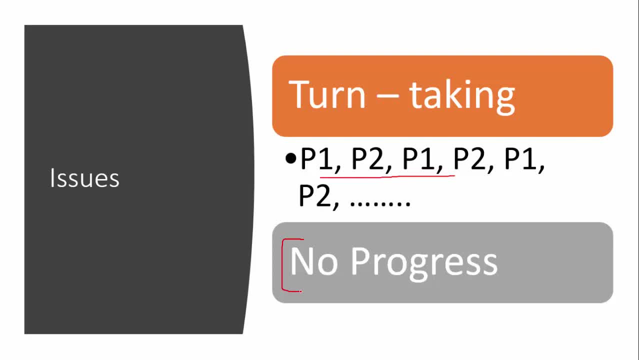 So in this case mutual exclusion is ensured. So we have seen that either P1 is entering or P2 is entering, So mutual exclusion is ensured. Bounded weight is ensured. One process's turn is a little more after the other, So the weight is limited to the turn of the next process. 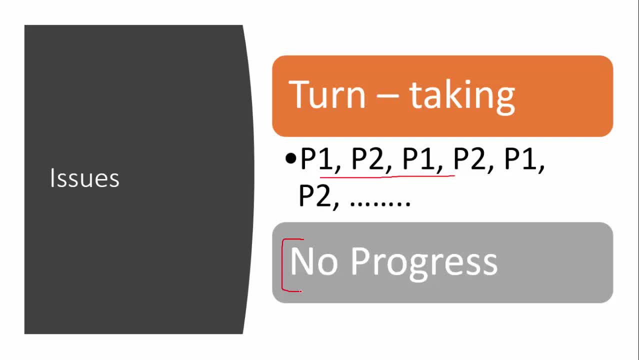 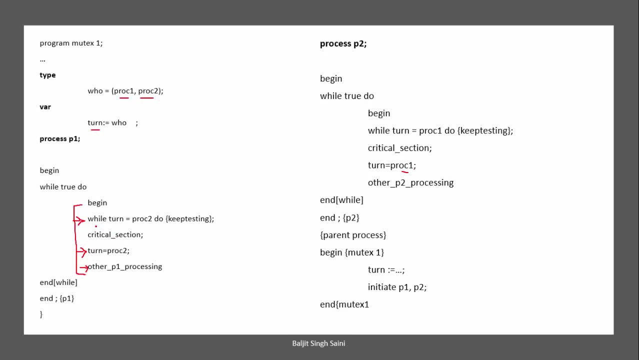 But there is no guarantee of progress. Now how will that happen? For example, let us suppose P1 was running Okay, It enters the critical section And then it gives the turn to process 2.. What is the turn? Process 2.. 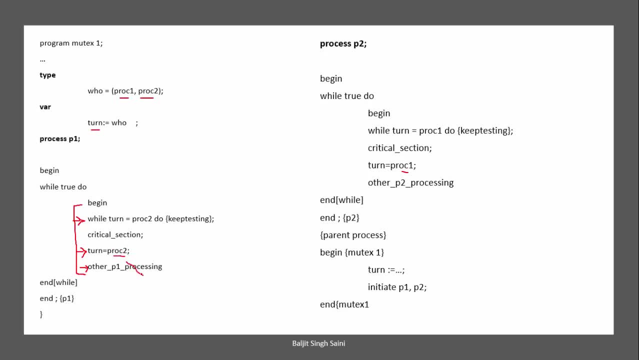 And now, after this line, P1 is terminated. P1 has given the turn to the process and it is terminated Right Now for P2,. what is the turn? Process 2. Right, So this will be false. It will be able to enter the critical section. 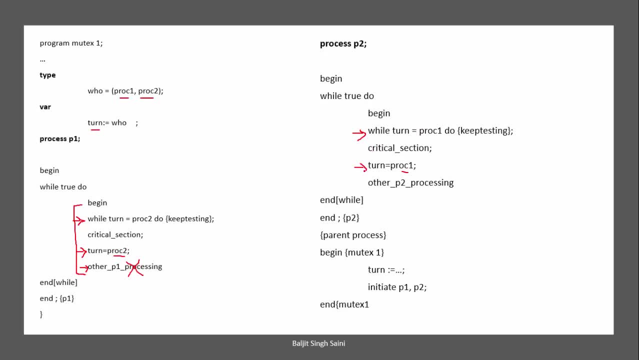 Or it will sign P1. But P1 is not in the system now. Now, if P2 wants to enter the critical section again, will it be able to do so? No, Because process 1 is not there And process 1 will never be able to change the value of the variable. turn back to process 2.. 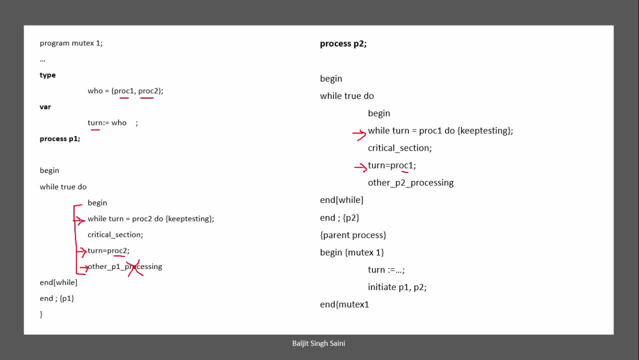 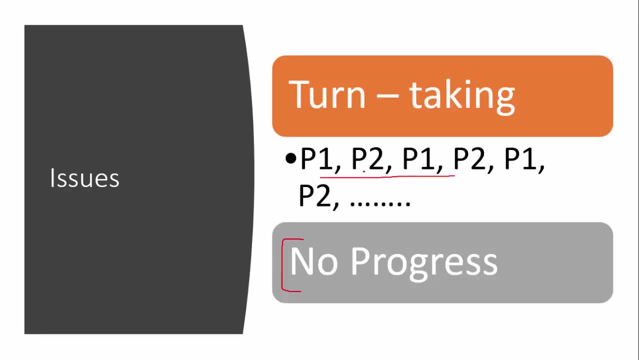 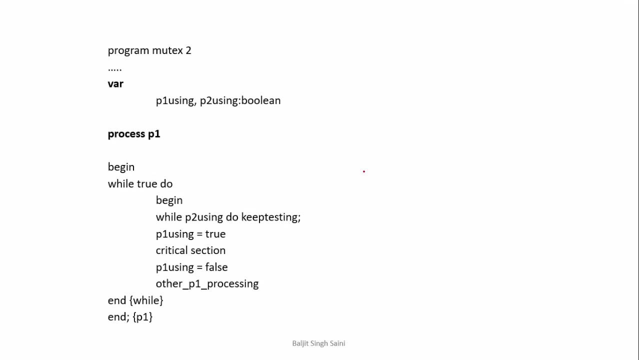 So P2 will not be able to enter the critical section, Even though it is the only process which wants to do so. Okay, So this does not ensure progress. One more example. So in this case, we are just going to modify the algorithm. 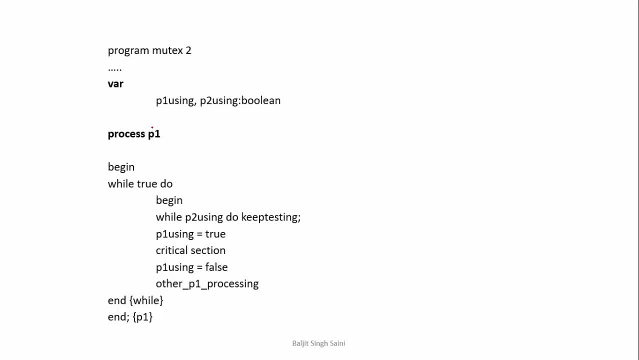 Now we are not going to take the variable turn, But we are going to take two variables: P1 using and P2 using. Both the process will have their own variables, And P1 using and P2 using are both Boolean variables. Boolean means that the process wants to enter the critical section. 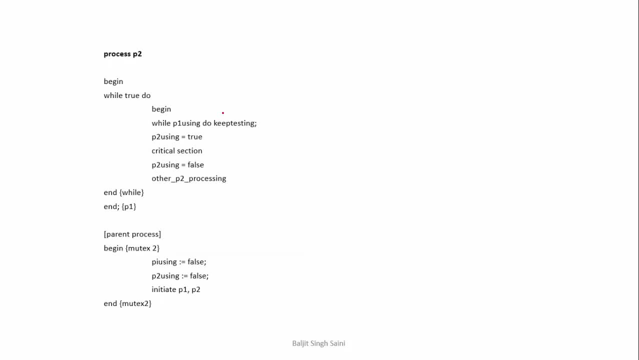 False means it is not interested to enter the critical section. So what is the initial value of both False Means? none of them is interested to enter the critical section. Right? So now we have written this code parallelly in the next slide. 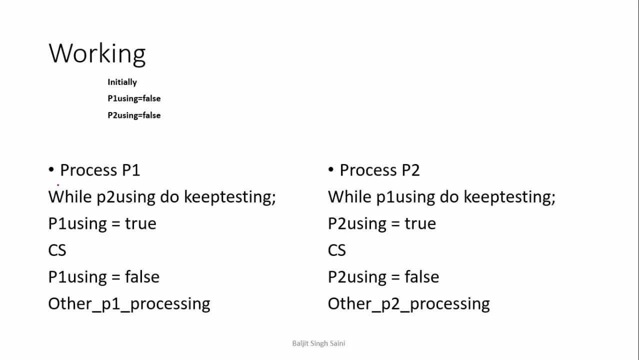 Okay, This is the code, Now what they are doing. Let us suppose P1 runs first While P2 using. Is P2 using true? No, It is false initially. So while P2 using, do keep testing. If P2 using is true, then what does P1 have to do? 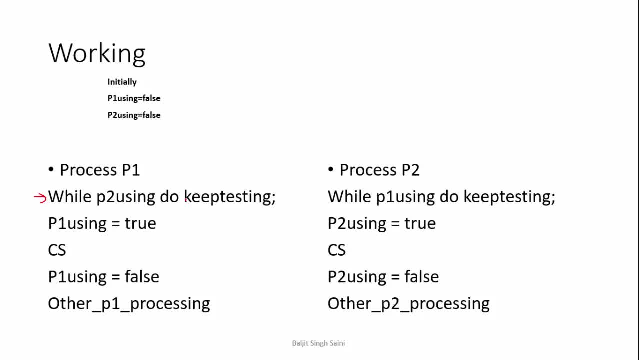 Keep testing Means, if one process has checked whether the other process wants to enter the critical section, Is it interested? Then it itself will not do so. So what will P1 do? It will initiate itself in the keep testing phase, Right? 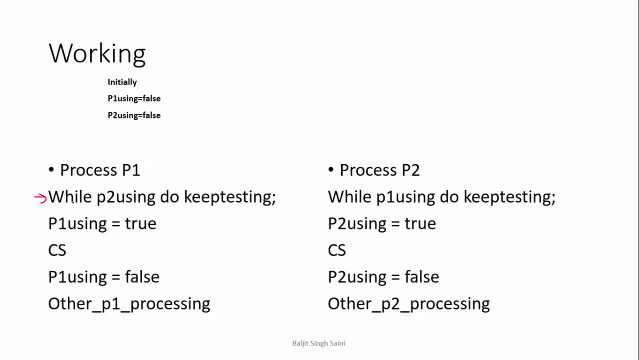 But since the value of P2 using is false, This means this condition will be false. Then P1 will itself change the value of P1 using to true. So P1 has changed the value of P1 using to true And it enters critical section. 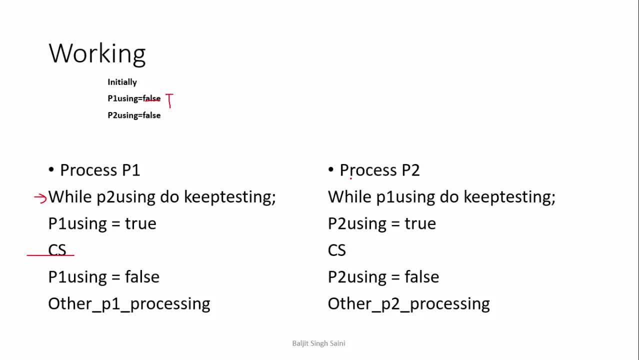 Now, once it is inside the critical section, If process P2 also wants to enter the critical section. So what will it do? It will check while P1 using. So P1 using is true. now Do what? Keep testing. So P2 will get stuck in the while loop. 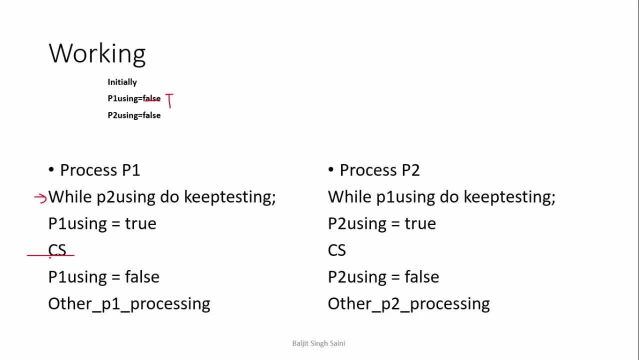 The moment P1 comes out of the critical section, It will change the value of P1 using to false. So what will it do? again, False. P2 was stuck in this while loop. Now, immediately this condition while P1 using. It is what. 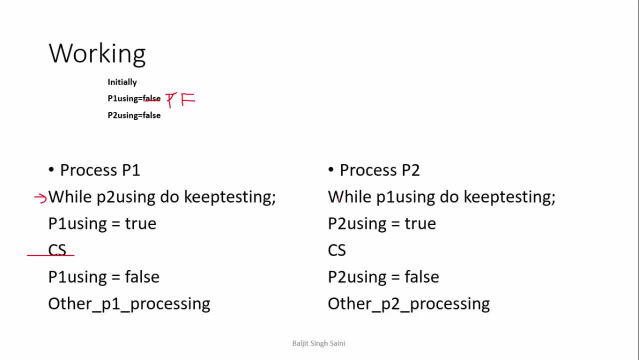 False. now This will become false. It will come out of the critical This while loop And will enter the critical section By changing its own value to true. Now what is the problem? Can you identify this? What is the problem in this? 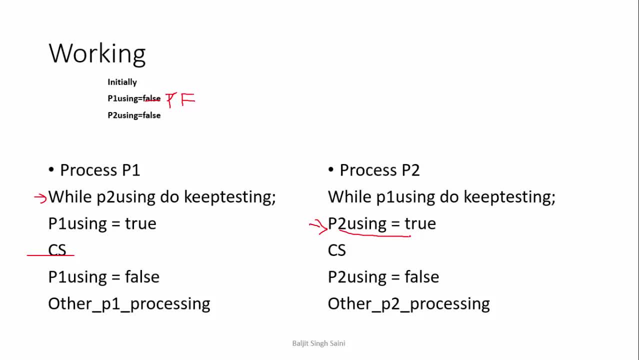 Yes, It does not ensure mutual exclusion If both of them comes at the same time, Exactly same time. The scenario till now was fine Because they were coming at different times, But let us suppose that Both the process start executing at the same time. 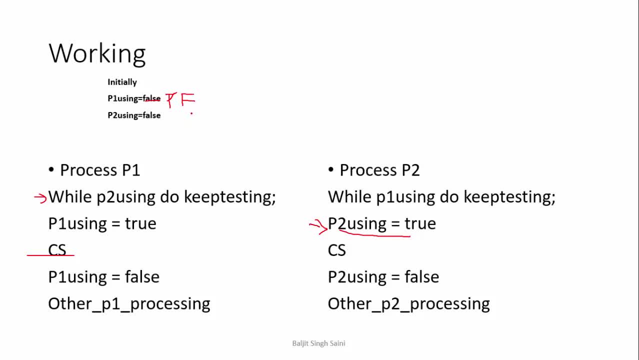 Then initial value of both the variables, P1 using and P2 using, is false. Both will execute this line at the same time. So what P1 will do While P2 using? What is the value of P2 using False. 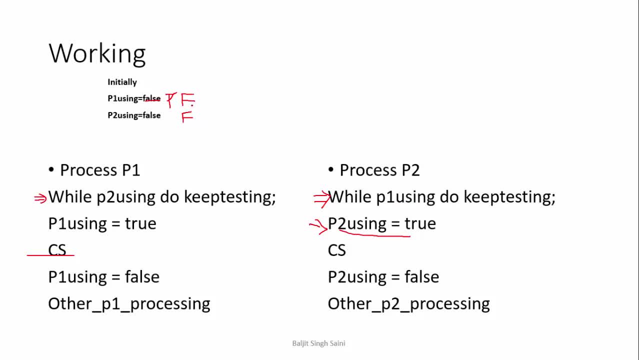 Check while P1 using. What is the value of P1 using False, So both will assume that the other one Does not want to enter the critical section. What is the value of the other one? False So means if the other one is not interested. 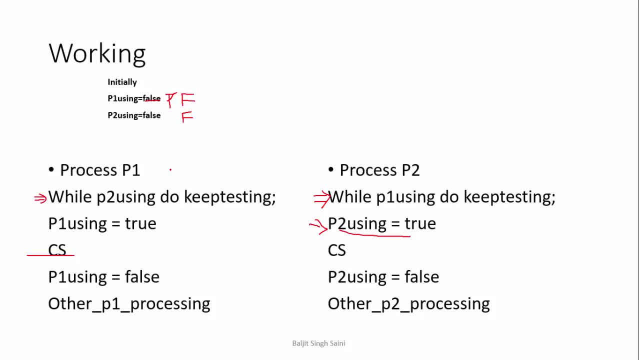 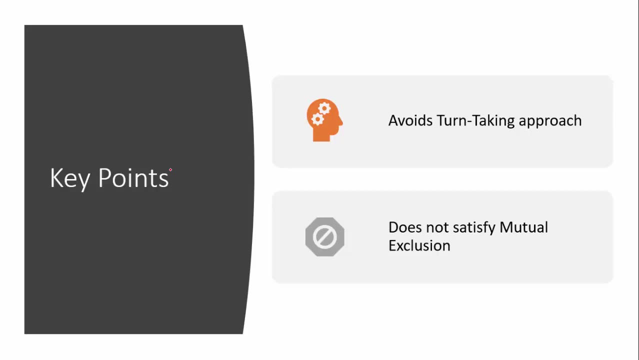 Then what will they do? They themselves will change the value to true And enter the critical section. So this solution will fail if both the process Starts to execute at the same time. Okay, So this avoids turn taking, But it does not satisfy mutual exclusion under all conditions. 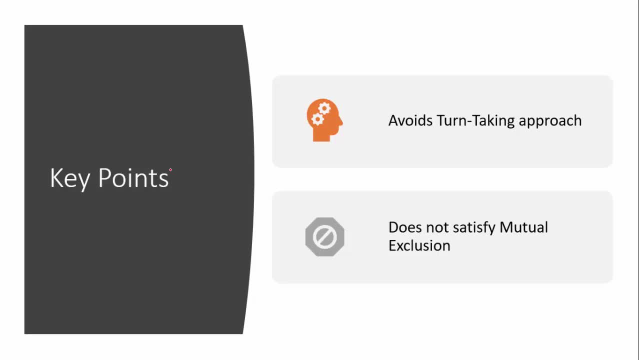 Okay. So remember that They will give you certain Solutions Where you need to tell whether Mutual exclusion, Progress And bounded weight Are satisfied or Not. So now one last algorithm: Peterson solution. This is the algorithm Which satisfies all the three requirements. 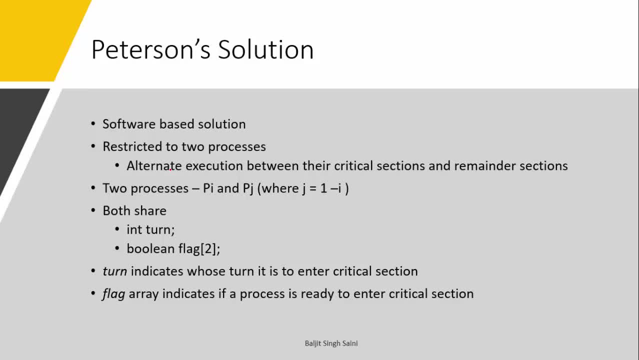 Okay, There are some important points to note down. First one is It's a software based solution. Second important point: It is restricted to Two process only. So this solution can work Only if there are Two process In your 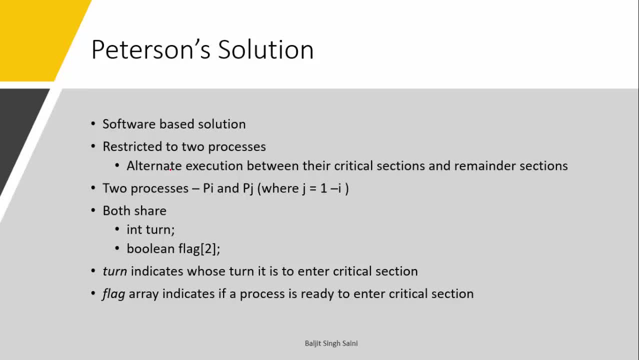 System. Okay, So this solution Can work Only if there are Two process In your System. Now We will Note Those processes By P I And P J Where the relationship is. 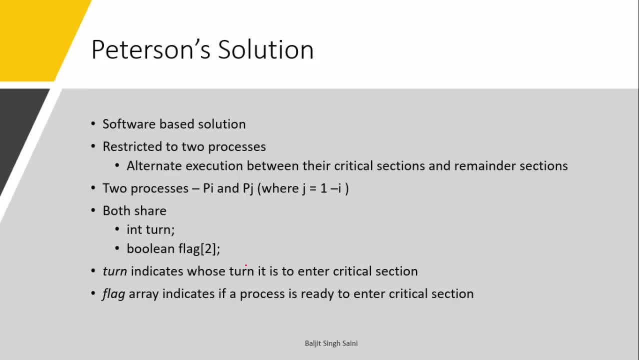 J is equal to One minus I. So if I Donate One of them As P Not, The other will be P One. Both the process Share Two variables: One is Turn And another is. 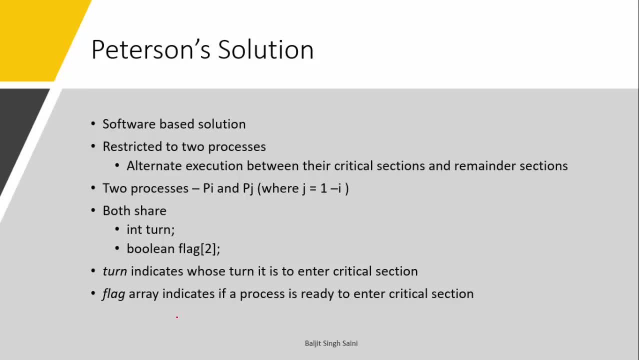 Flag P, Not As Well As P One Or P I And P J. Whereas Turn Is A Shared Variable, Okay, Turn Indicates The Process To. 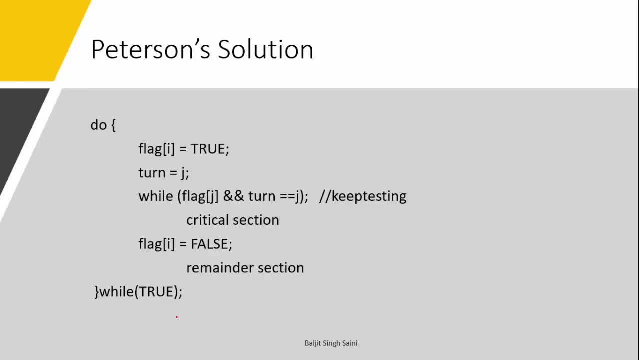 Enter The Critical Section. So What A Process Will Do? It Will Set Its Own Flag To True When The Process Up. Now Flag True. So 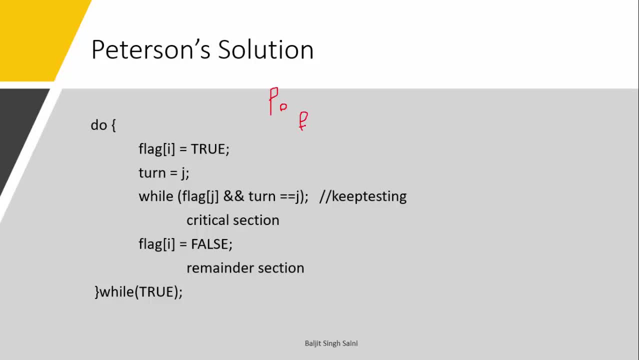 For Example, Let Us Suppose That P Not True, Okay, And Will Give The Turn To J, Turn To One: Okay, Our Flag True And Turn. 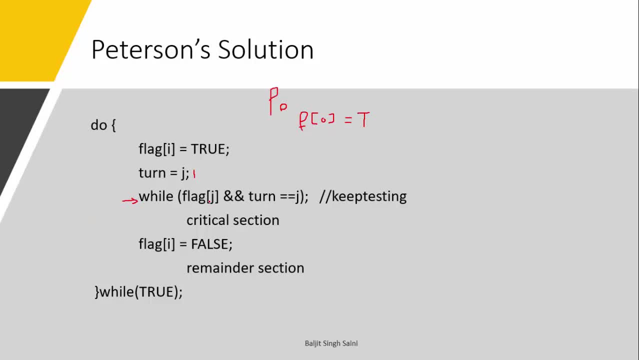 To The Other Process. Now Check This Condition. While Flag Of J Is Also True And True, Okay, So Since Only P Not Is Executing, 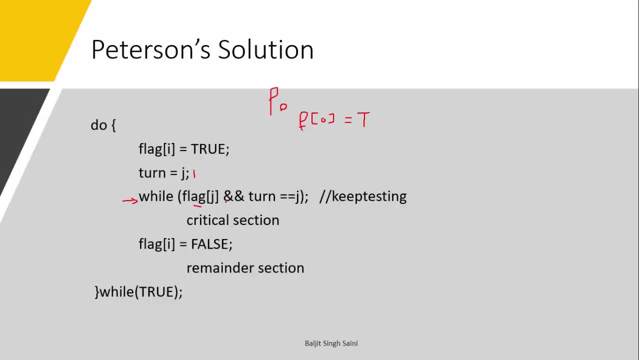 At This Time. So Flag Of J Will Be False Initially, Sub Flag False Now P1. If P1. Comes At This Time, What It Will? 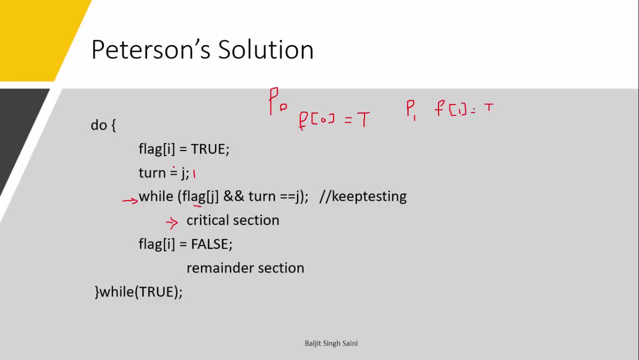 Do, It Will Set Its Own Flag To True. Flag Of One True. Now Flag True And Turn Flag Of P0. Its Flag Is True. 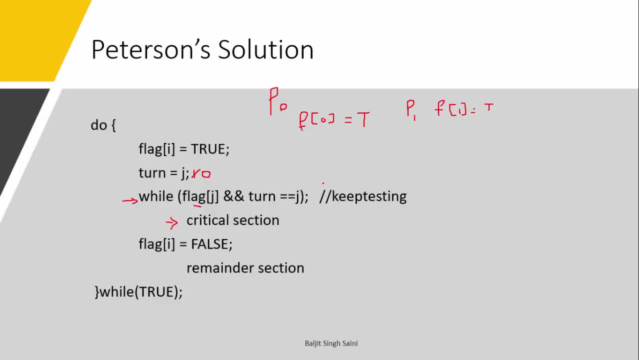 We Set Turn Of P0. So Flag Is True Of P0.. Turn Of P0. Then This Condition Will Be True, So P1. Will Be. 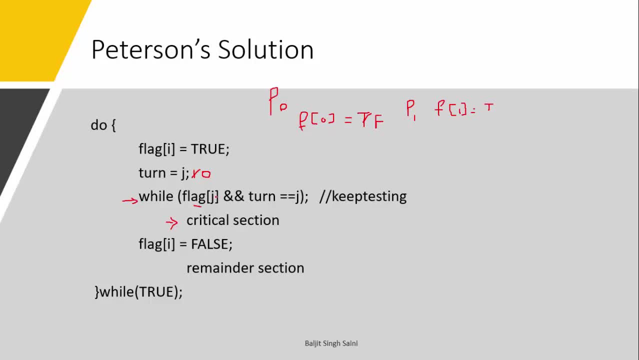 False Since P1. Was Stuck In The While Loop. Now Flag Of Not Is What Flag Of P0. Is What Now? It Is False. 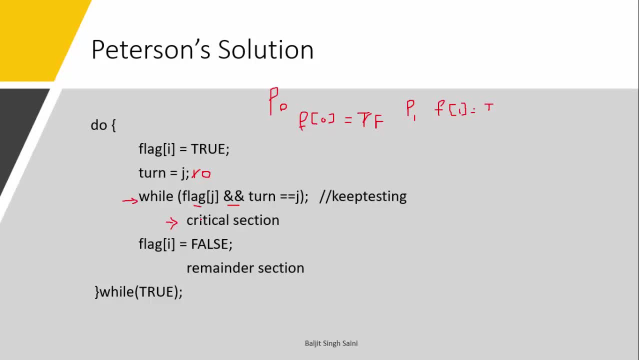 So While 0. And P0. Is True Of P0., Turn Of P0. Is True, So P0. Is False. Now P0. Is True Of. 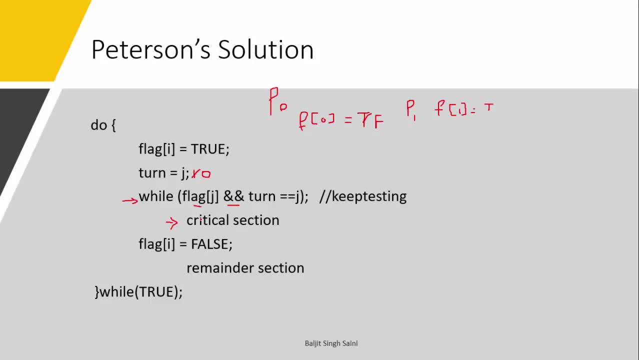 P0. Of P0. Of Turn Of P0. Of P0. Of Turn Cause, But Dependent of Of His Concordance, To Note For Next And 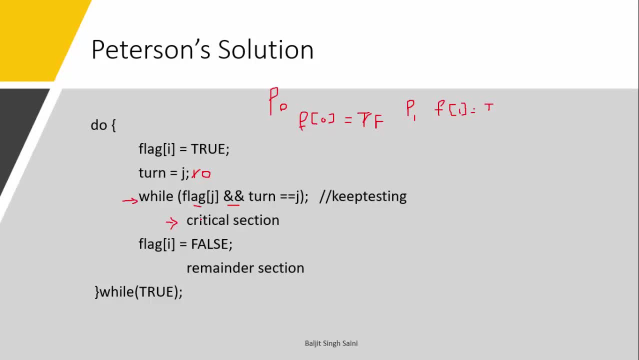 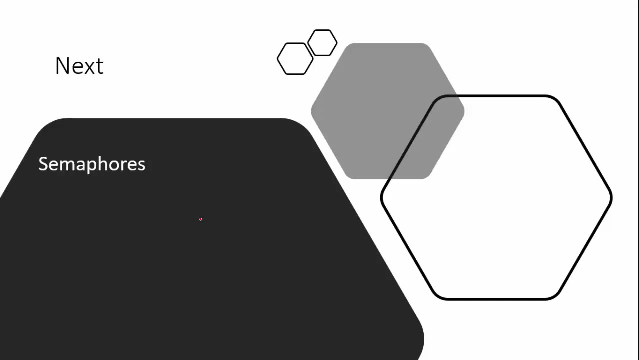 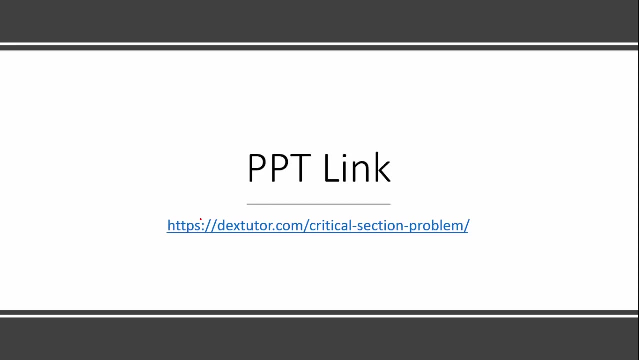 One Of Up return Summer Of постоянно Solution. A Request From A Of A Of So Of Is semables. the dpt is available on this link. so if you like this tutorial, please do share. and subscribe. see you next time. take care.